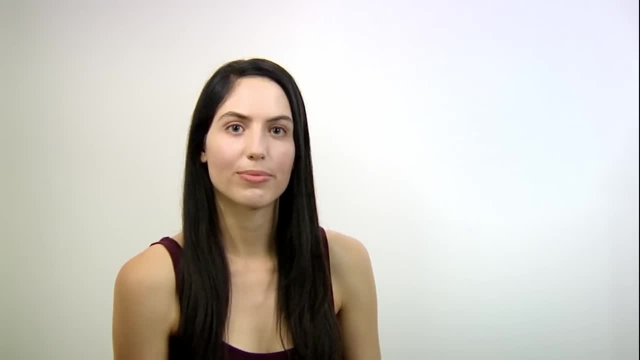 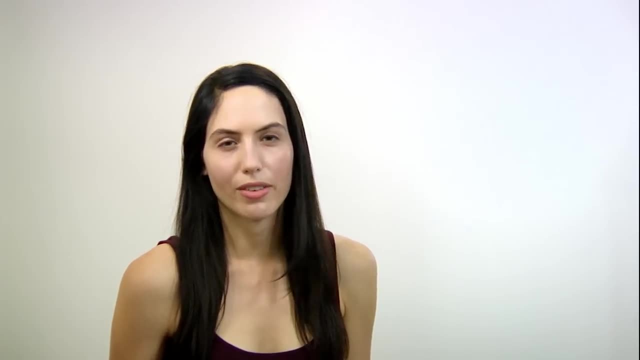 is taking that y and giving you back x. Why would you want to do this? Good question, I don't know, but your teacher wants you to, so let me show you how to find the inverse function. So what you'll already need to know is how to tell if something is a one-to-one. 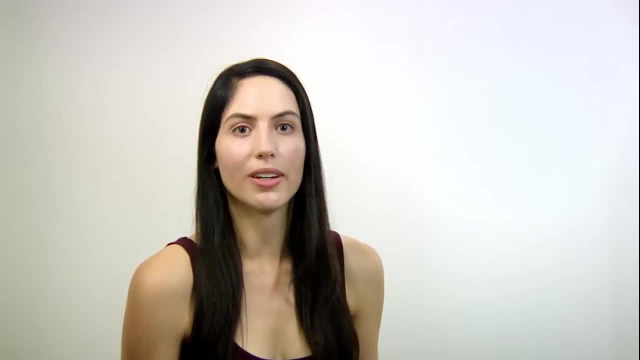 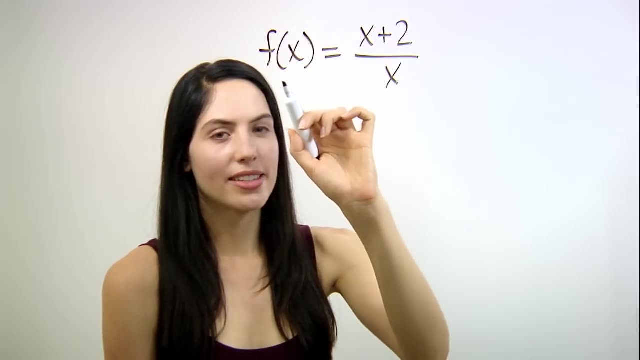 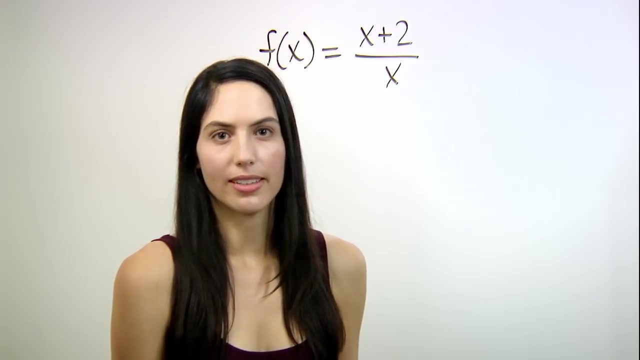 function. So for every x value you only have one corresponding y value. Okay, so say you have a function like this: f of x equals x plus 2 over x, and you need to find the inverse, if it exists. Of course, for this function, we also need to keep in mind that x cannot. 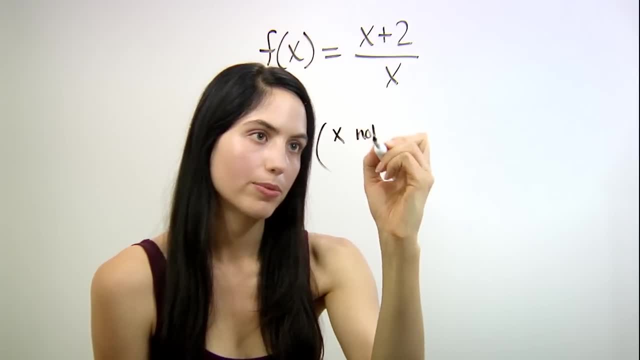 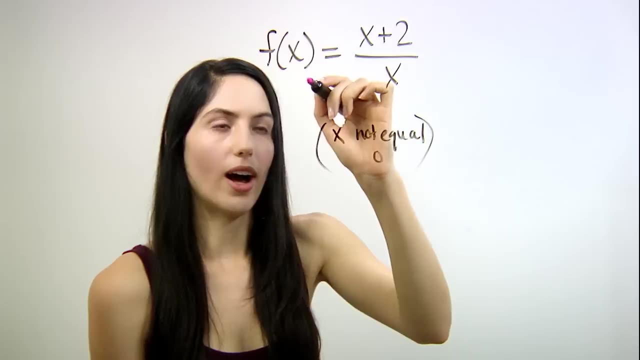 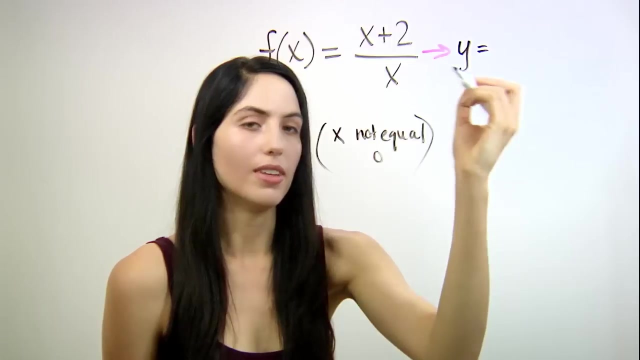 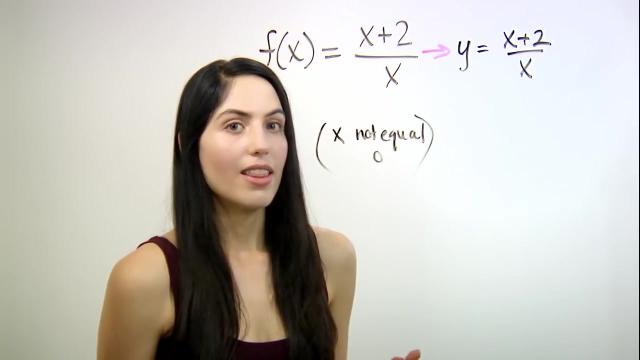 equal zero. because we can't do that, The first step is just to rewrite f of x as just y, So we would just have y equals x plus 2 divided by x. Then- this is the most important step. you need to swap x and y, So you switch. 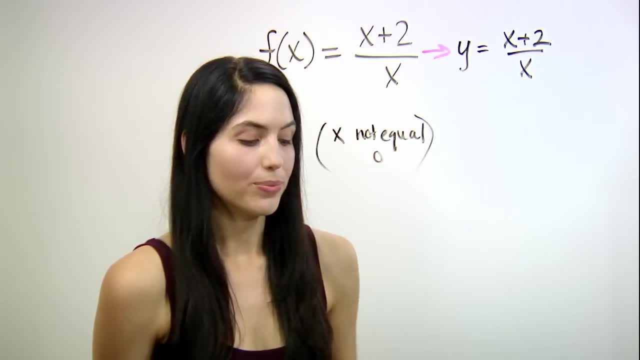 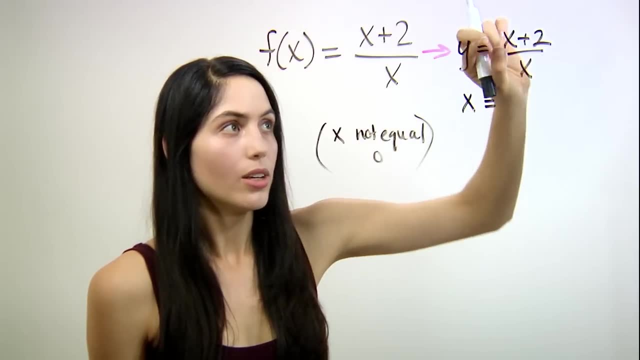 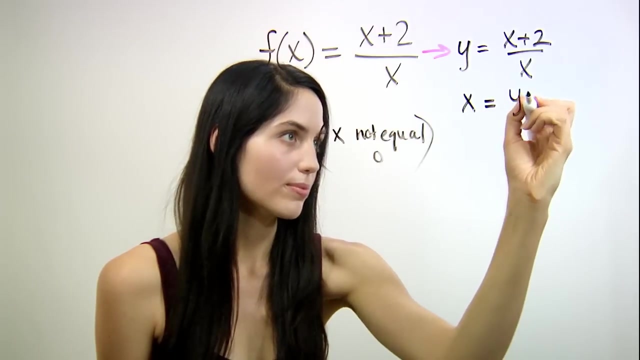 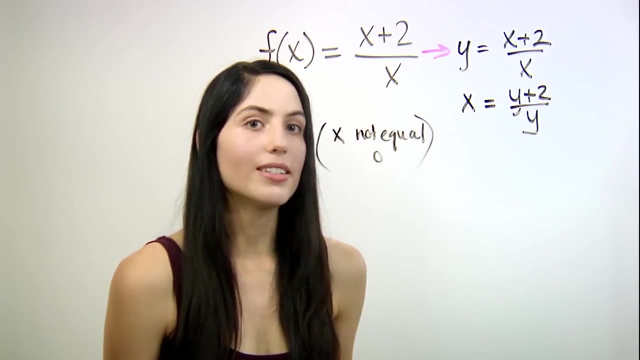 x and y everywhere they appear. So we would actually have x on the left side instead of y Here on the right side. replace x with y everywhere, So we would have y plus 2 divided by y. Last step you need to solve for y so that we're back to. 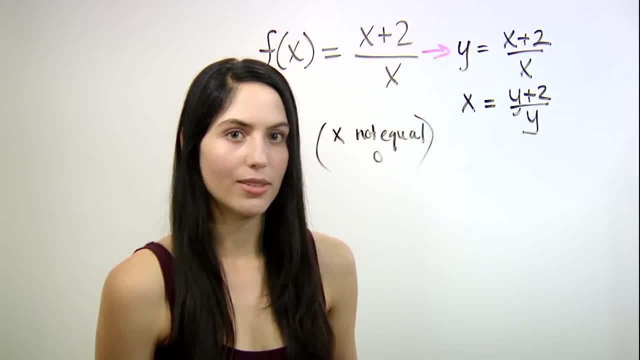 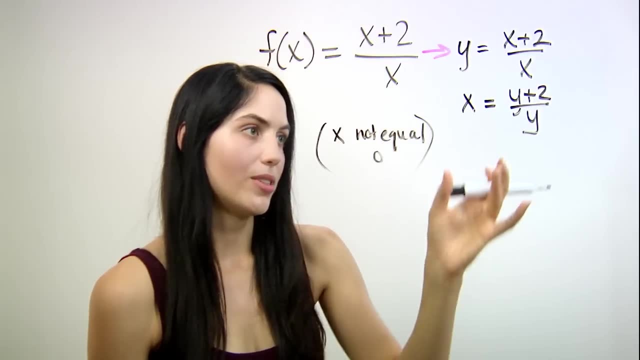 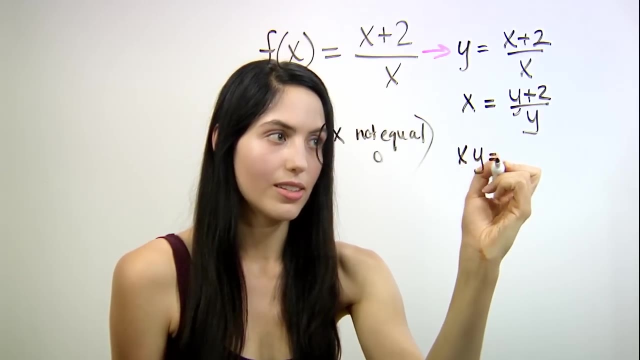 y equals with y alone on the left side. To do that, we'll need to clear this fraction. So you would multiply both sides by y to clear the fraction and then get in the next line: x times y equals just y plus 2, because we've cleared the y. 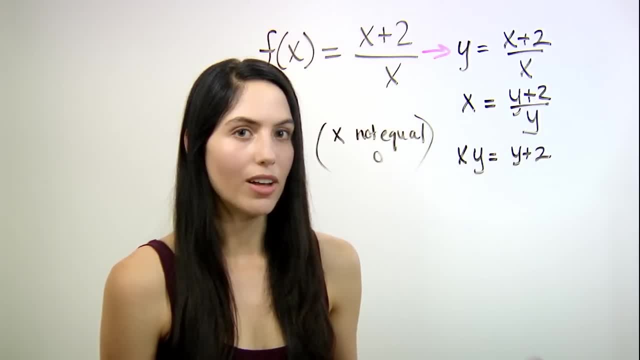 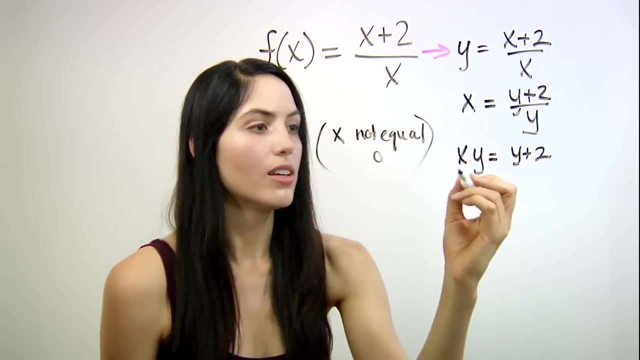 Then if you want to get y alone, you'll need to have all your y's on one side. So why don't we just bring this y over to the left by subtracting it from both sides, So you get xy minus y equals just 2.. 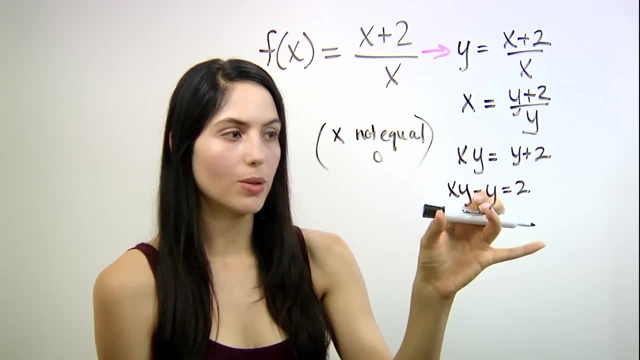 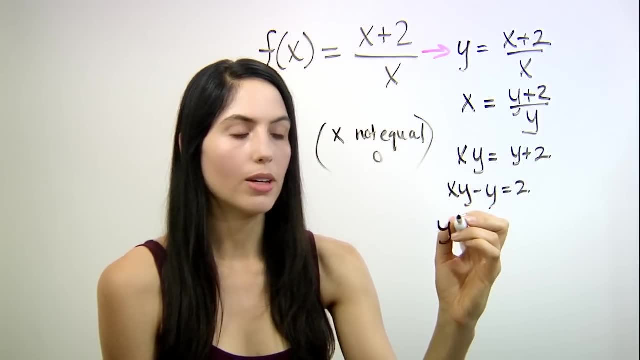 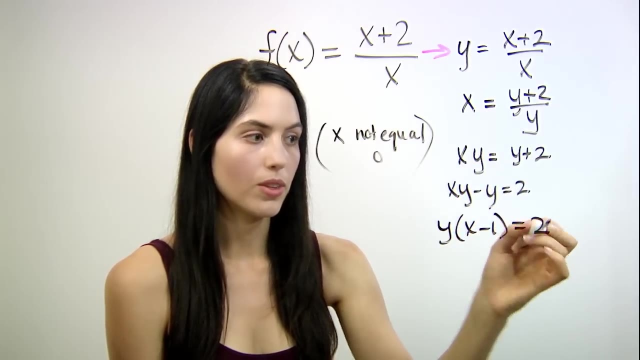 Now to solve for y. you only want y to appear once on the left side, So the best way to do that is to factor out a y, So you'd have y parentheses and what's left is x minus 1 equals 2.. 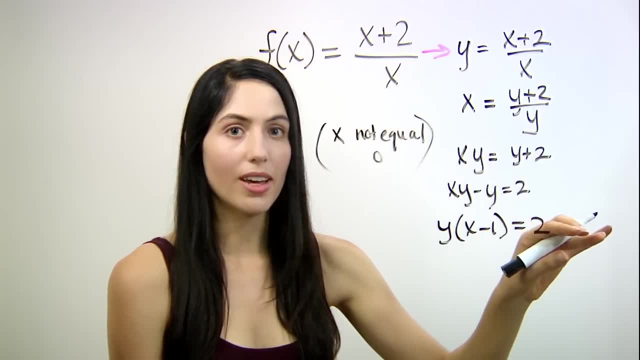 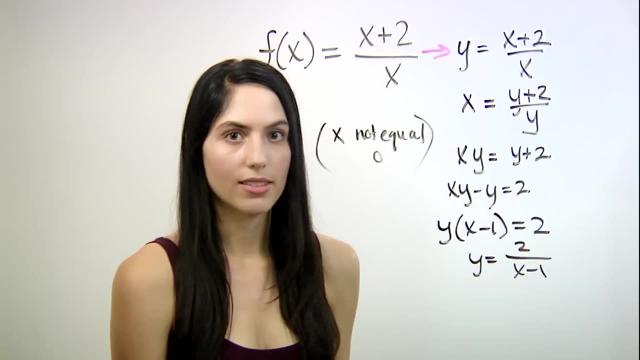 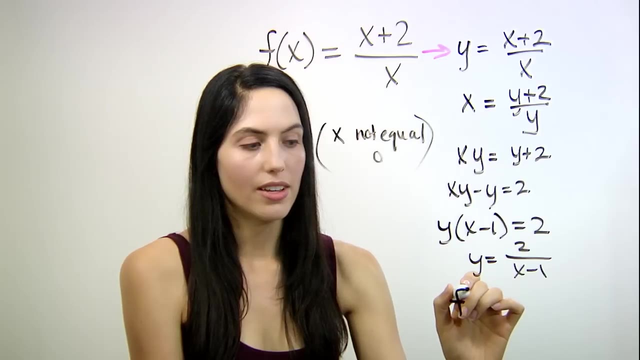 Final step: divide out the x minus 1 from both sides. So you have y equals 2 divided by x minus 1.. To write this as a function we would use inverse notation f. inverse with a negative 1 superscript of x equals the. 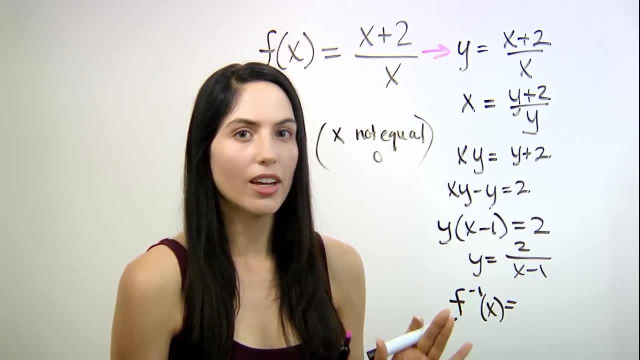 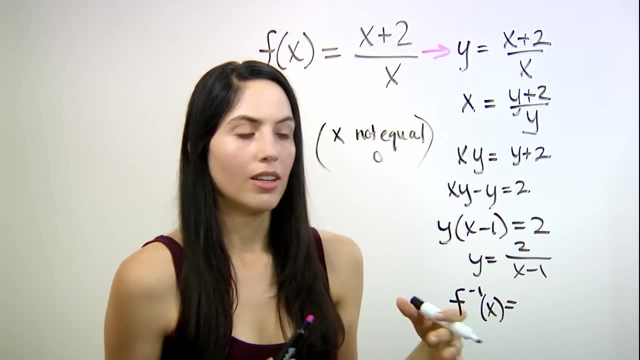 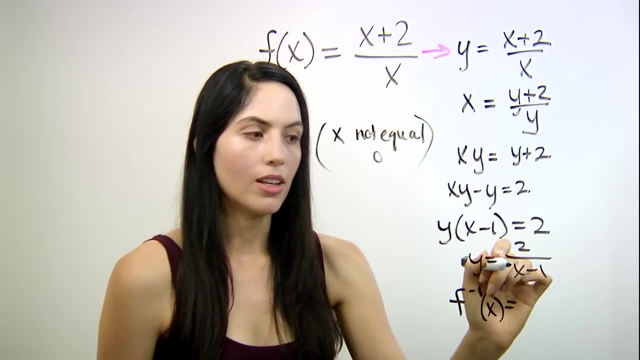 expression. But first you have to check that this is actually a function. Sometimes it's just a relation and not a function. Is this a function? It is because for any one x value we plug in, there's only one corresponding y. 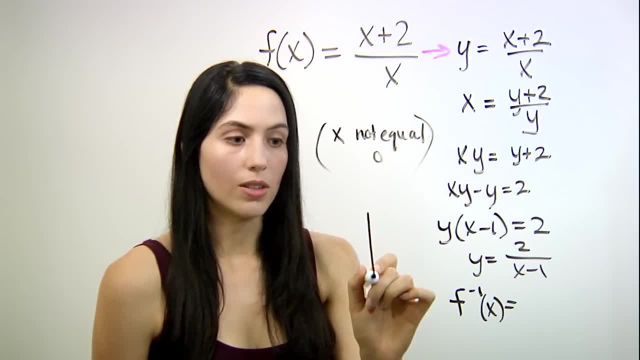 And if we look at the graph of this function, as you know, it would look something like this: So if you did the vertical line test, you'd get y equals 2.. So if you did the vertical line test, you'd get y equals 2.. 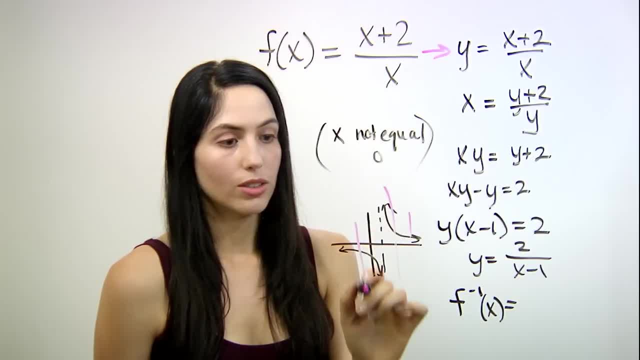 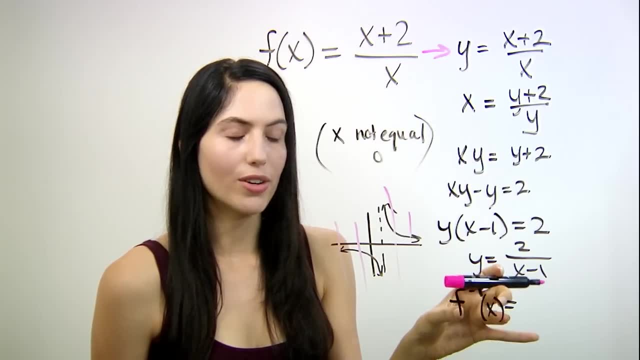 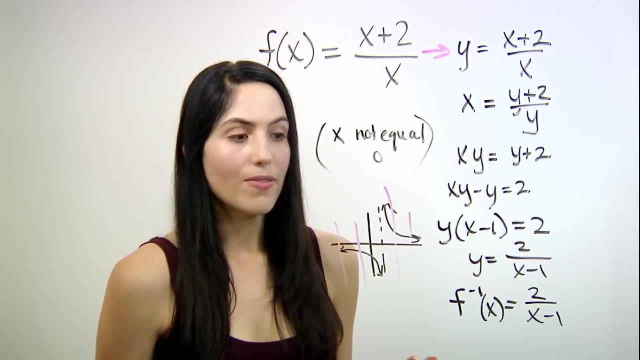 So if you did the vertical line test, you'd get y equals 2.. We also know that the union is just 1. before we tests the universities and we're außer Grace operation, which is b, We can check that the Y function is İn. 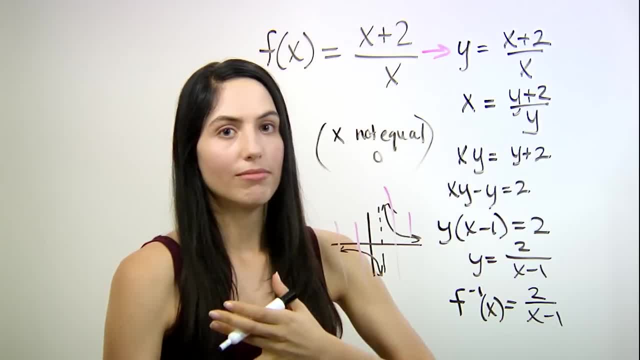 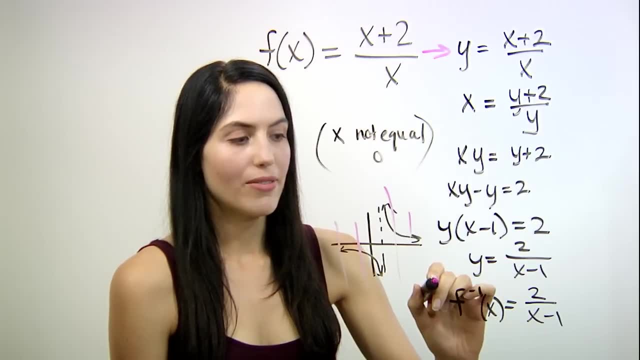 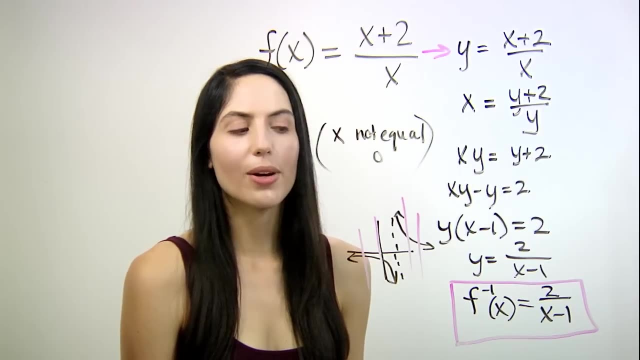 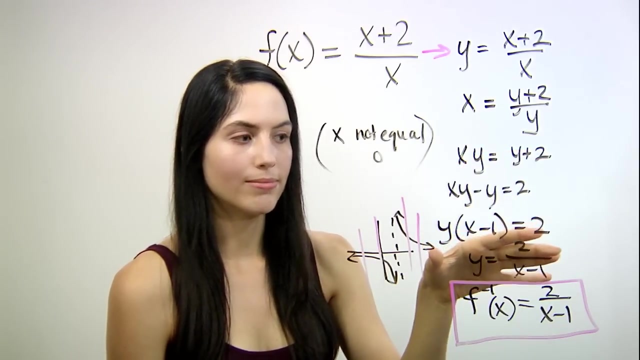 if you will. So this must be gone over the date. this of x equals 2 over x minus 1.. So this one magically worked out. but some things to look out for: where you may not have an inverse function and your inverse function doesn't exist is if you have a y squared somewhere here in your 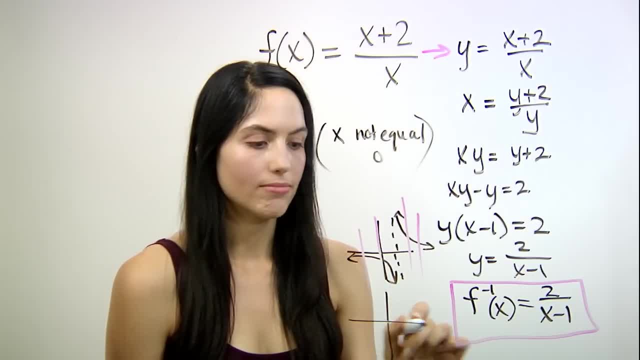 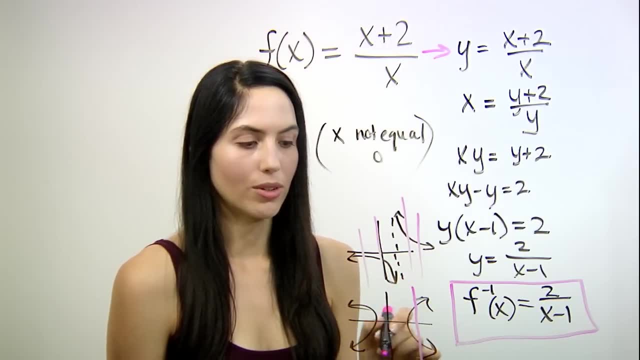 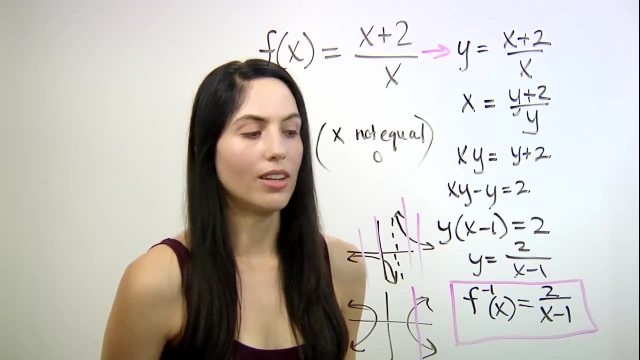 equation or you have a graph that could look something like this, where if you do a vertical line, it would cross more than once, might cross twice. you wouldn't have a function in that case, so you wouldn't have an inverse function and you would just say that your inverse function doesn't exist. I hope this video.